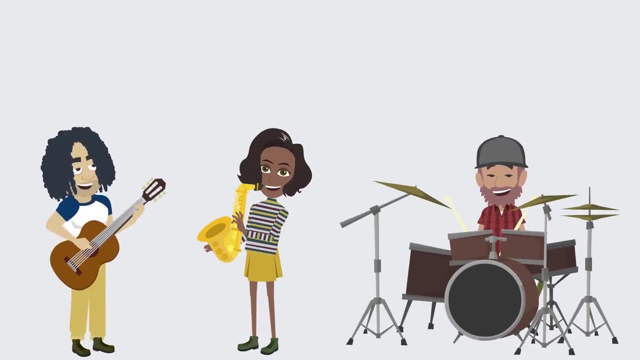 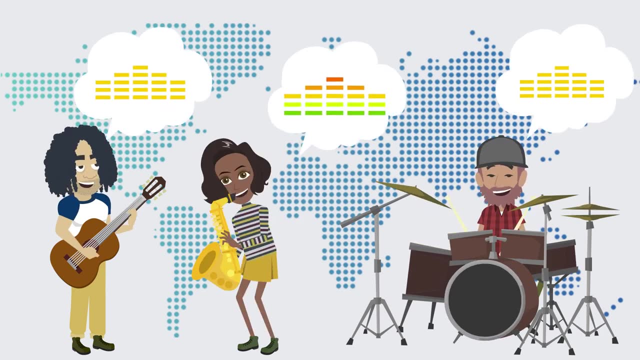 Over time, more and more musical instruments have been developed, and with the huge advances in the digital world, so too has the actual sound of music. In general, the tempo is faster, the beat is livelier and the volume is higher. 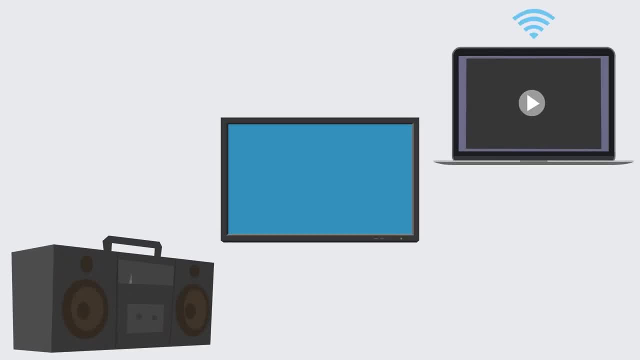 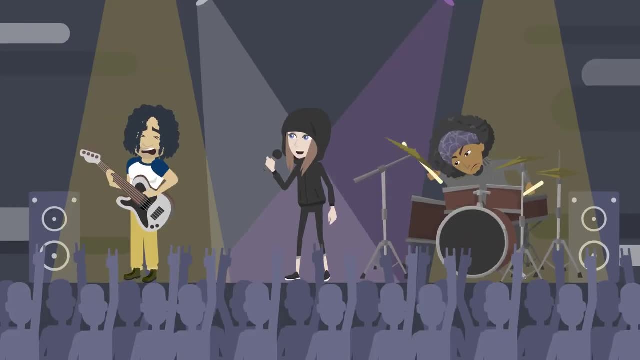 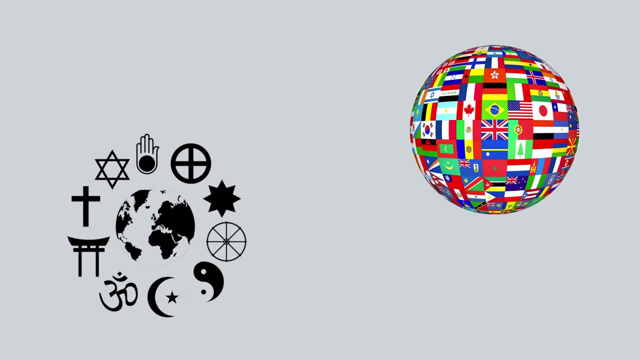 We can hear it on the radio, on the TV, online, on the street, in bars and clubs, at concerts. We all have access to music. somehow, Music bonds people to religions, to cultures, to friends, family, loved ones. 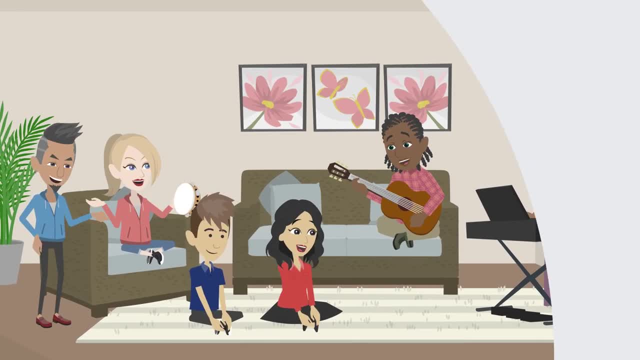 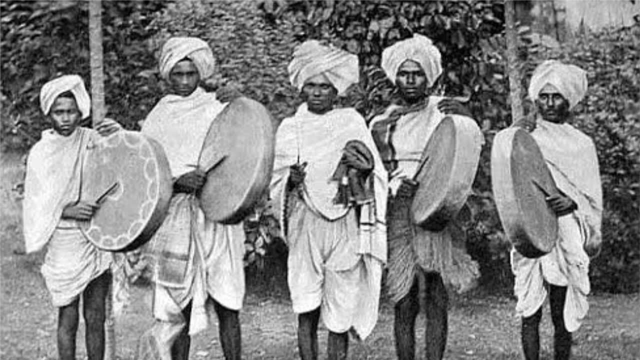 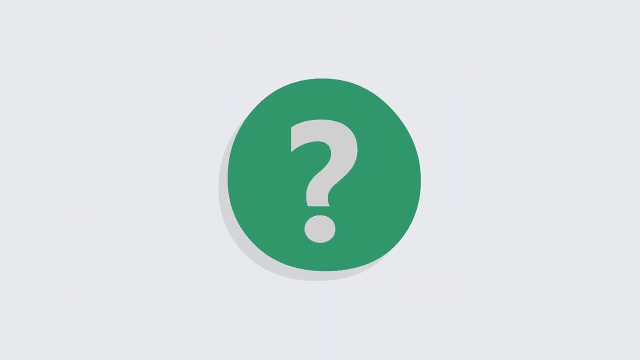 to memories. It is an essential part of society today, As it was hundreds of thousands of years ago, when tribes also got together to socialize and entertain. I mean, there's no party without music, is there? How do music trends change, though? 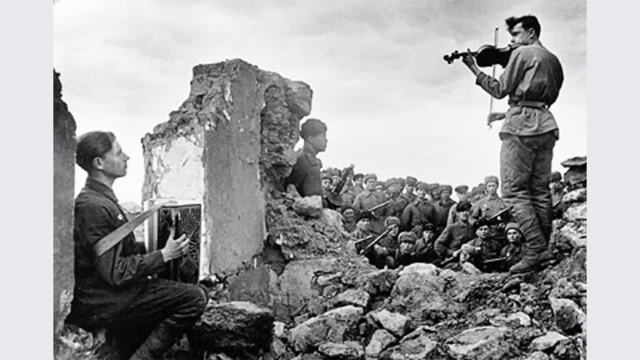 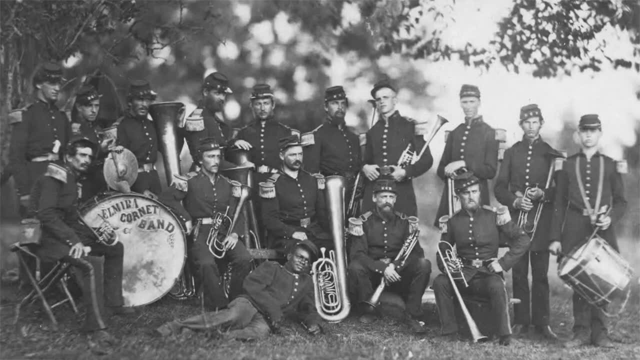 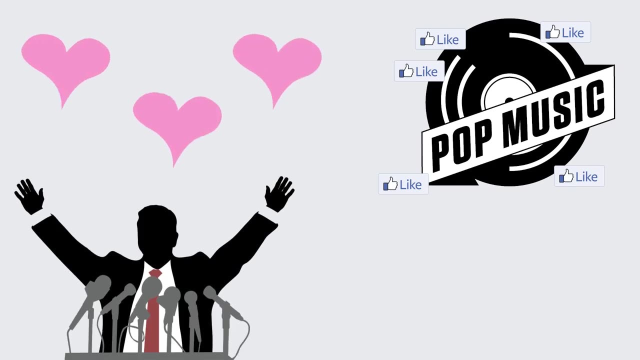 Well, they are significantly influenced by history. For example, during the war, most tunes told stories of people's struggles and hardships. Nowadays, most pop music is reliant on music. It is related to social media, politics, love and the way people feel about each other. 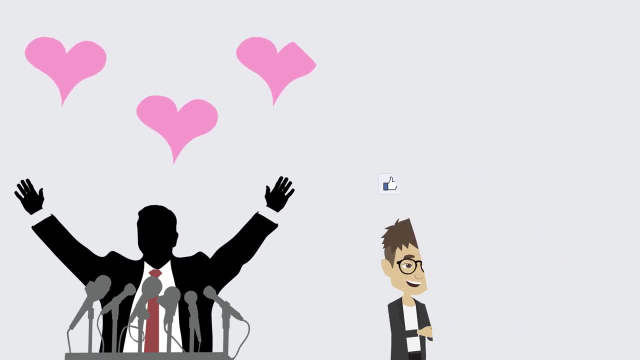 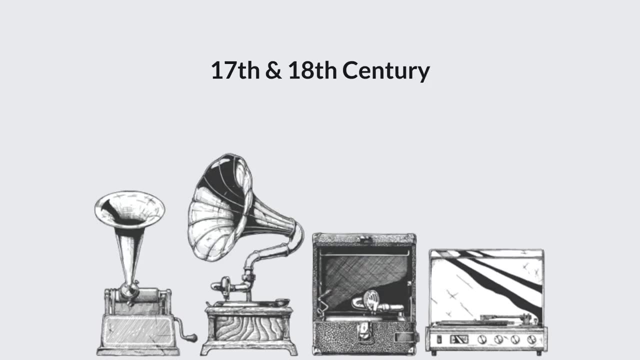 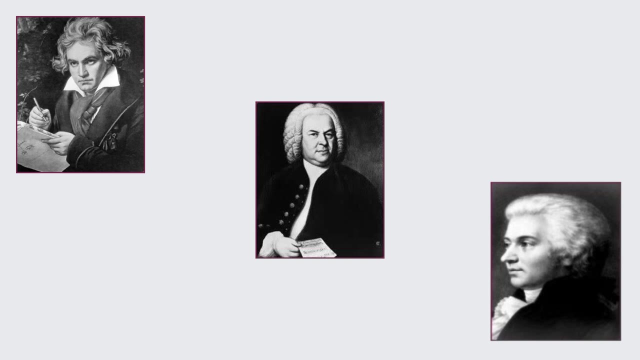 Because that's how society is shaped. We have to thank the great composers of the 17th and 18th century for their huge involvement in the evolution of music. Beethoven, Bach and Mozart are considered the top three masters of classical music. 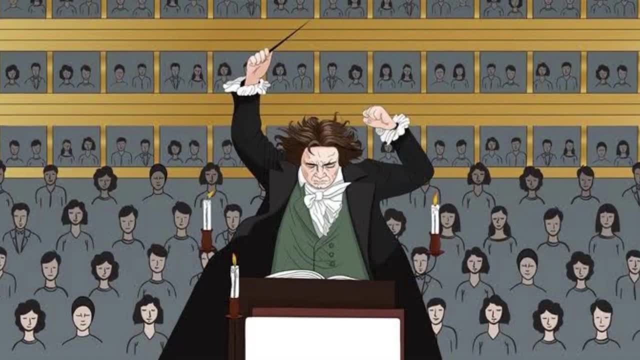 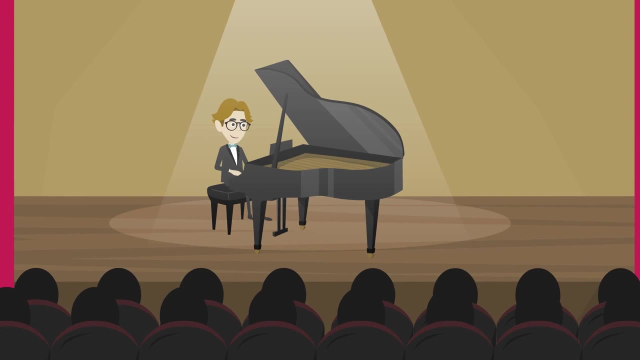 Interestingly, Beethoven suffered with music progressive hearing loss, but was still able to produce some of his most famous works during this time. Classical music may not appeal to the masses, but it actually helped to form the foundations of modern-day pop music. 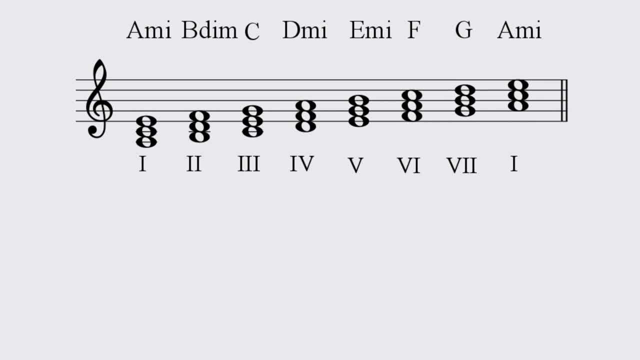 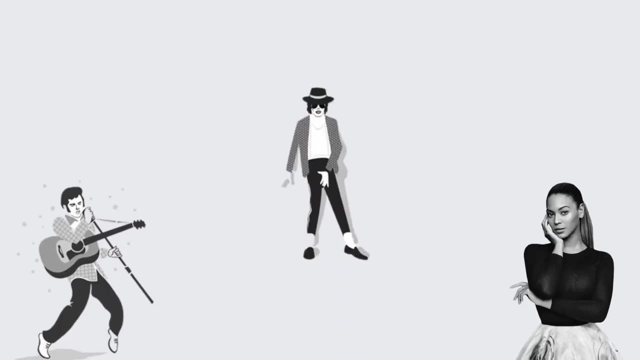 Most classical tunes are built from the seven tones of the major and minor scale. And yes, you guessed it, so too is pop music. Who would have thought that artists like Elvis Presley, Michael Jackson or Beyoncé would feature in the same sentence as Ludwig von Beethoven?